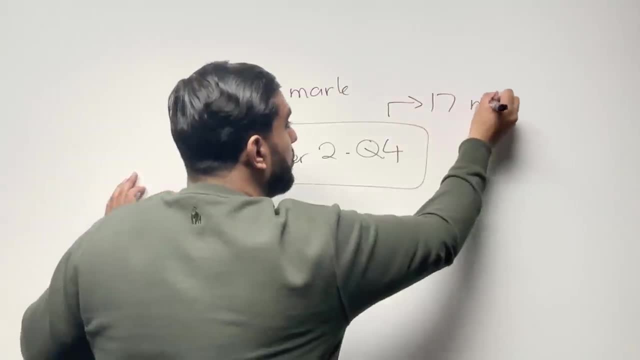 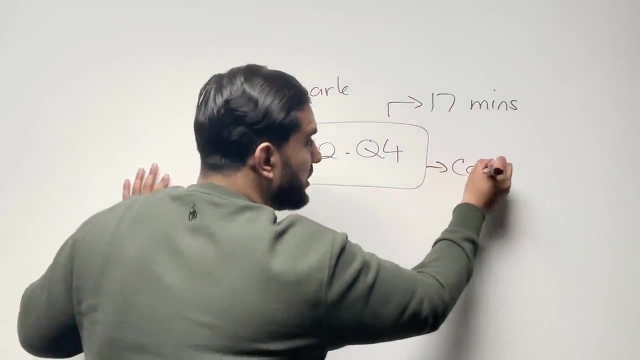 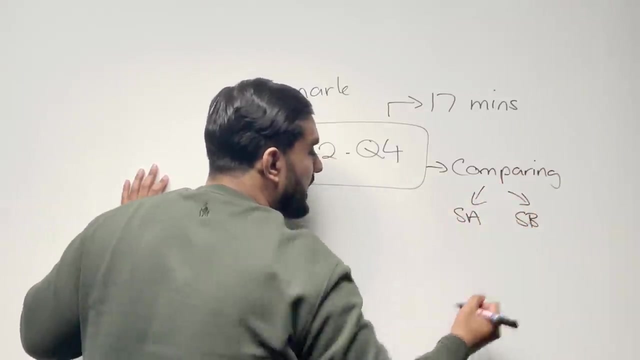 mark question and for a 16 mark question, we are looking to spend 17 minutes on this particular answer. and in this particular question, guys, we are comparing. Now, what are we comparing, guys? We are comparing source A to source B and we are looking at methods. Now, when writers talk about, 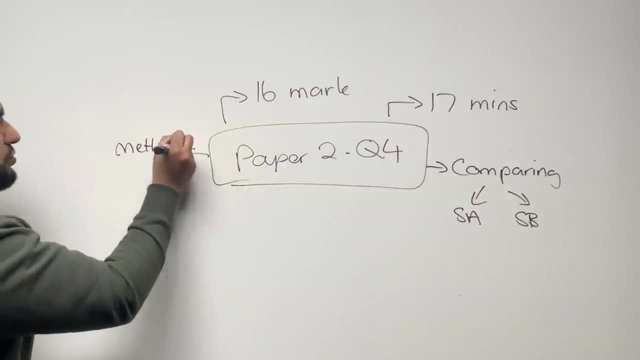 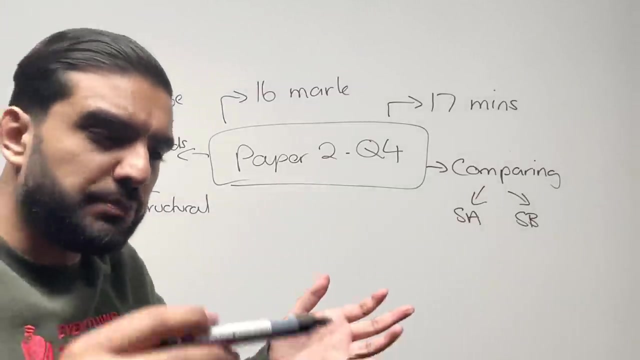 methods. guys, they are referring to two essential things: They are referring to language techniques and they are referring to structural techniques. Now, if you've made it this far in your English language exam history, So you've done paper one. question one. question two. question three. question four: question five: 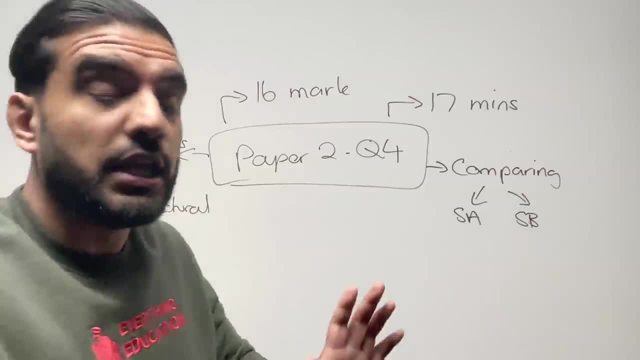 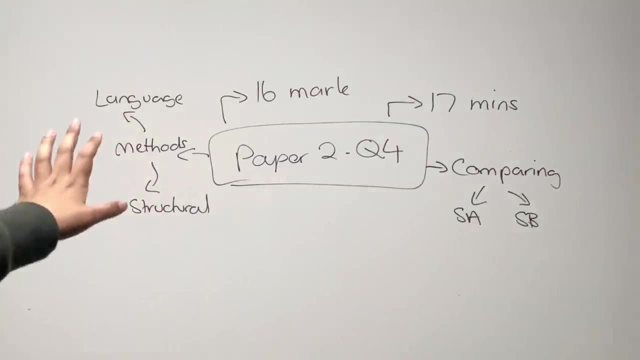 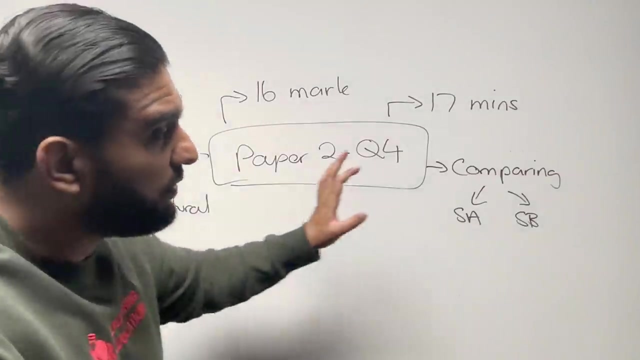 paper two, question five: one, two, three. This should be second nature. This should be second nature. You should know 100% what language and structure is. Now, guys, language is language devices, structure is structured devices. So we're comparing source A and source B. We've got 17 minutes. We've got 16. 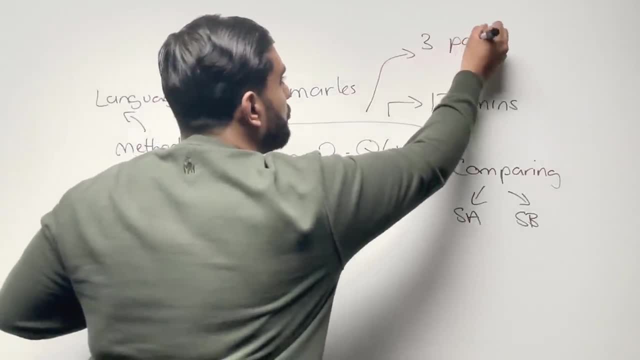 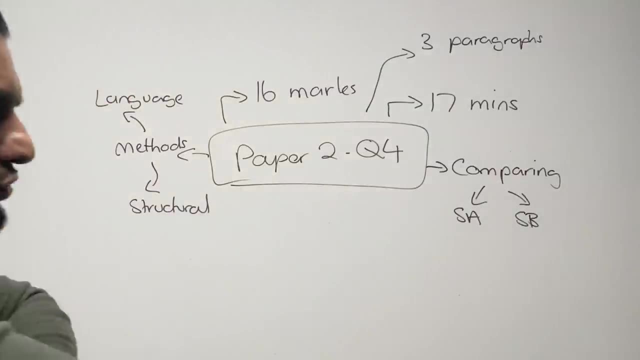 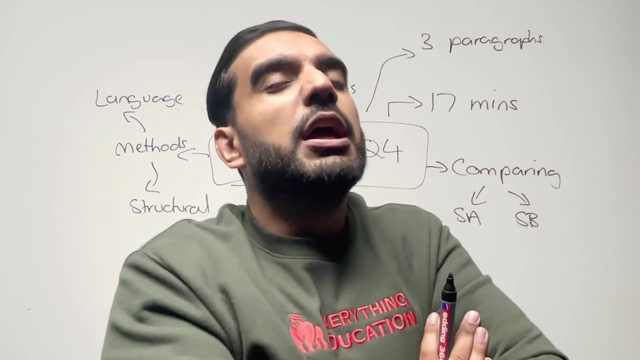 minutes Now for this question. guys, you are aiming to write three paragraphs. You are aiming to write three paragraphs, Now, what paragraph structure do we use? Do we use pretzel? Do we use pita? Do we use peel? Guys, we don't use none of them because none of them allow us to compare. Guys, none of them. 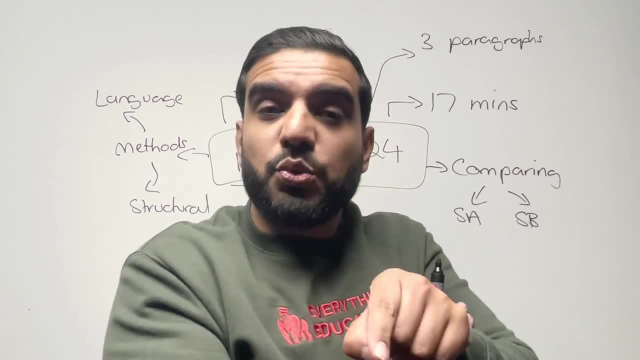 allow us to compare. Now I'm going to prove to you, when we look at the question, why the structure that I'm going to go over is a bulletproof structure, But the structure that I'm going to go over is a bulletproof structure. 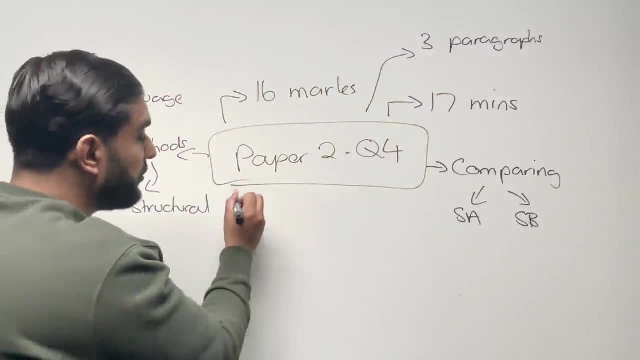 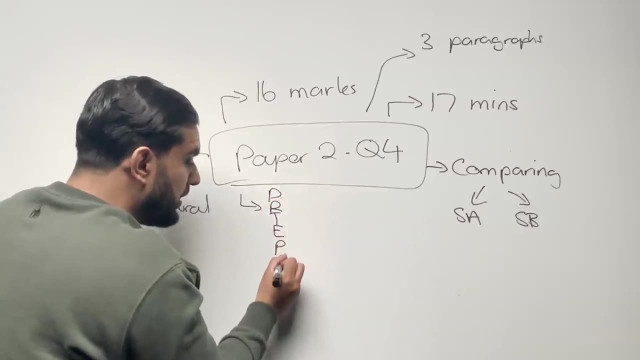 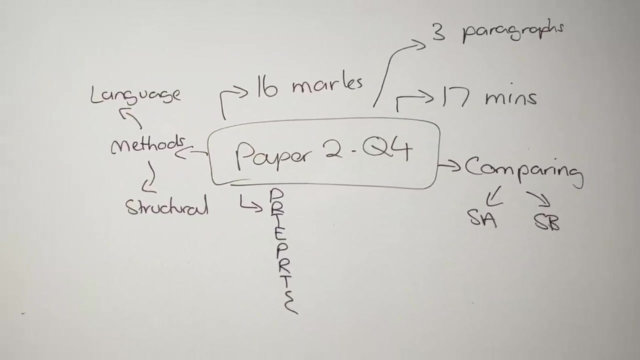 The structure that we're going to be doing, guys, is we're doing three paragraphs. right, We're doing three paragraphs. This is the structure of one paragraph. You got p? r t and e, p? r t and e. That is the structure. I don't know why I wrote it so squashed up, guys. I don't know why I wrote it so. 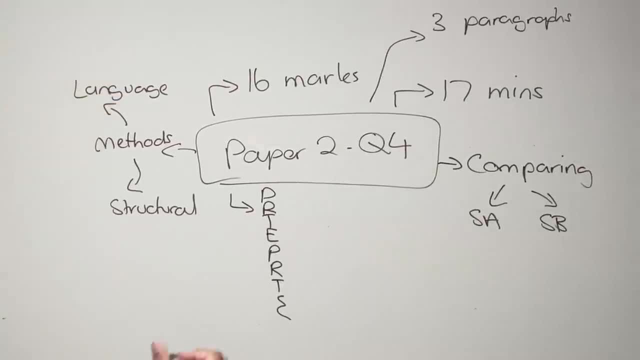 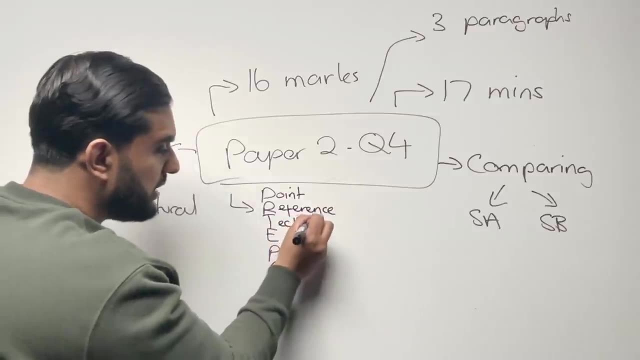 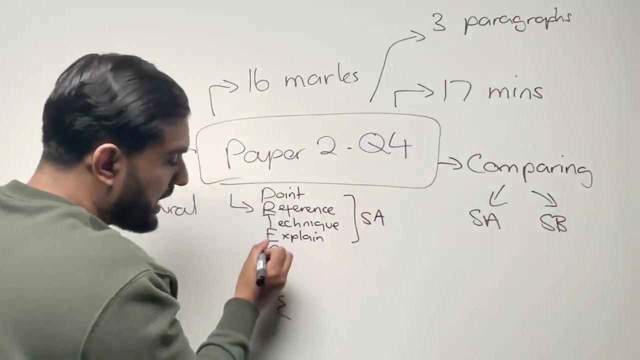 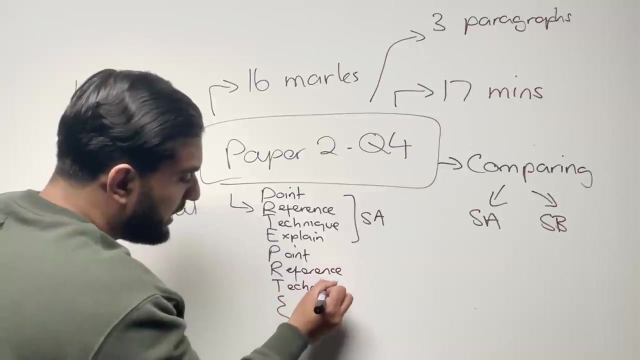 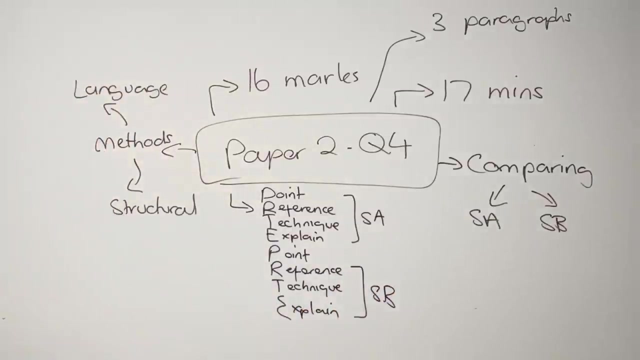 squashed up, But we are aiming for point, Guys, we are aiming for what. We are aiming for point: reference technique. Explain the effect. This is source a, Then we do our point, Then we do our reference, Then we give our technique, And then we explain again for source b. Now, at this point here, guys, 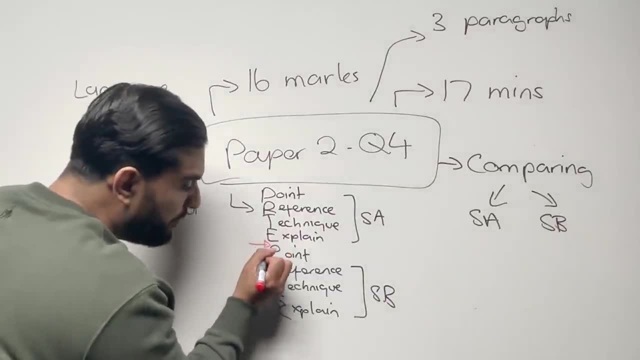 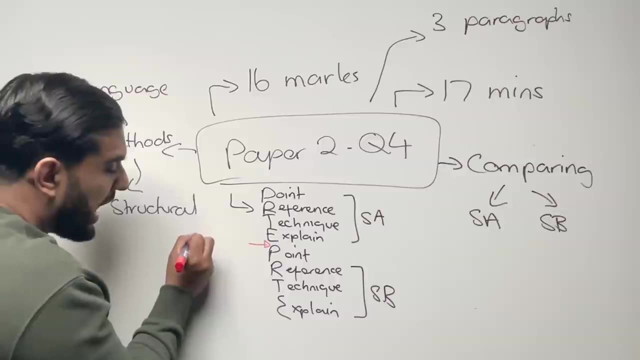 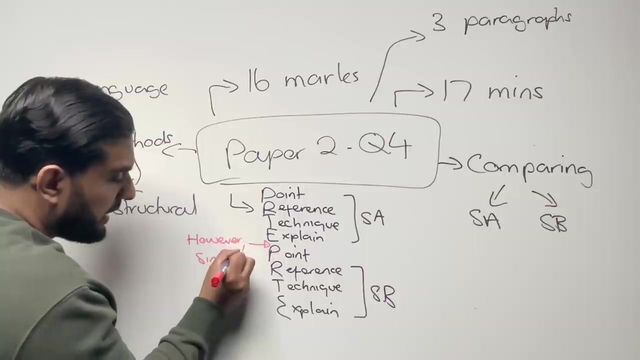 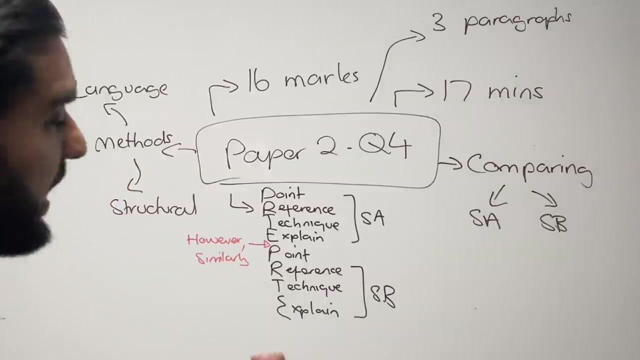 at this point here, before we move on to source b, Depending upon what we're doing, we either say something like, however, which indicates a difference, or we say something like similarly, which indicates a similarity. That's the first thing. Then, when we do our second, effect you want to make reference. 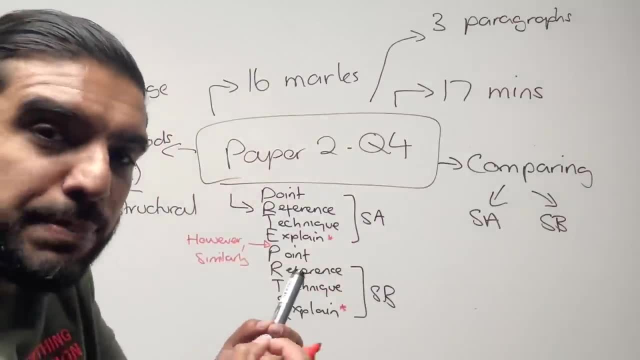 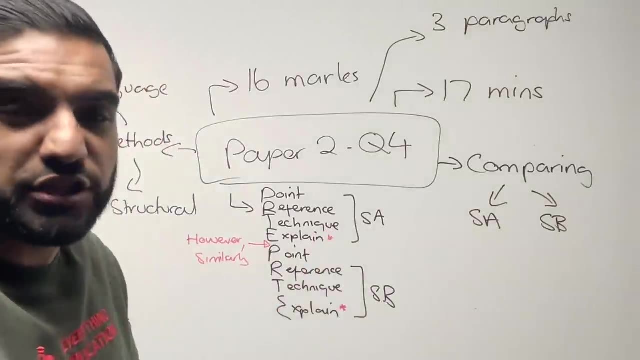 to your first effect, because you want to slightly bounce back and forth, Because, again, guys, we are doing a comparison, but that is the paragraph structure that you want to follow. Now, guys, what we're saying. sir, how am I going to be doing that? How am I going to be doing that? how am I supposed? 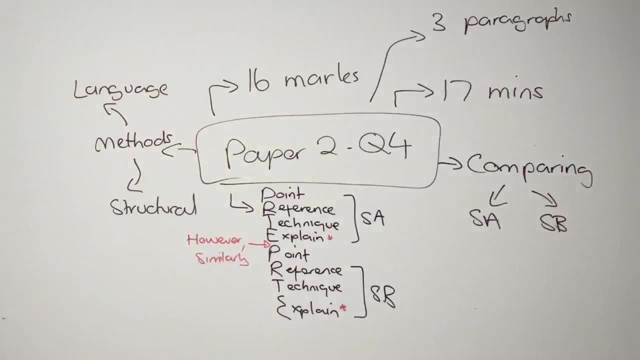 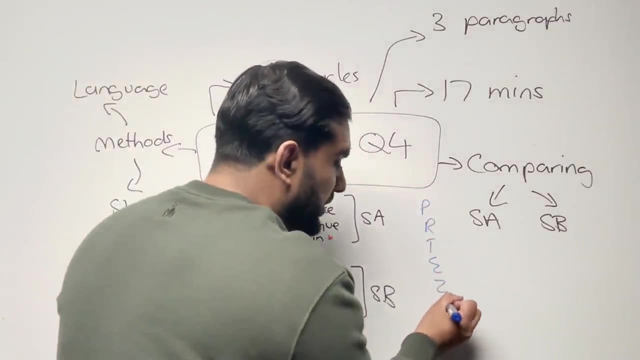 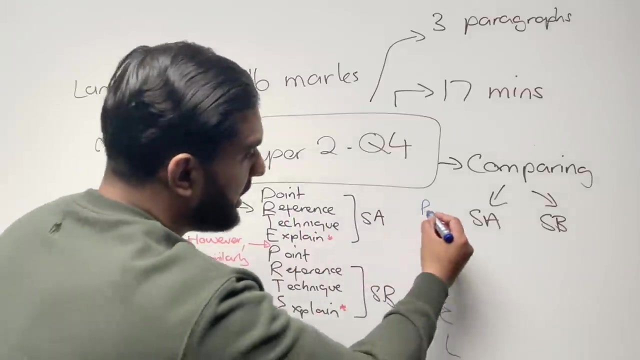 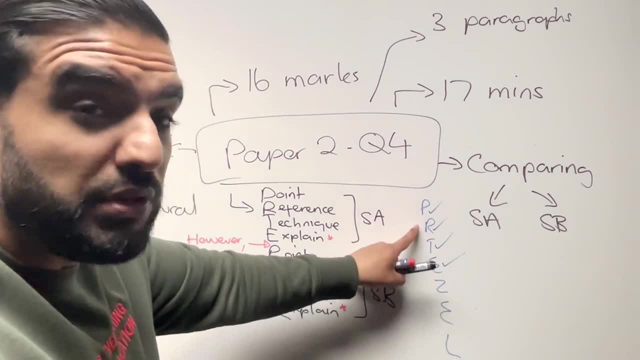 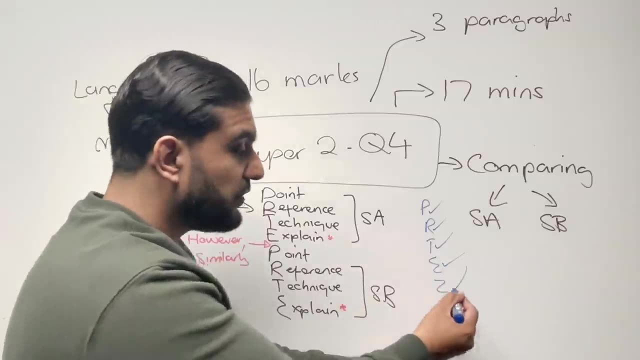 Now, rather than zooming in to the same quote, rather than zooming into the same quote, we're now picking out a different quote and a different technique from the other source. Then we're explaining the effect of the other source, The only thing that we are really adding. 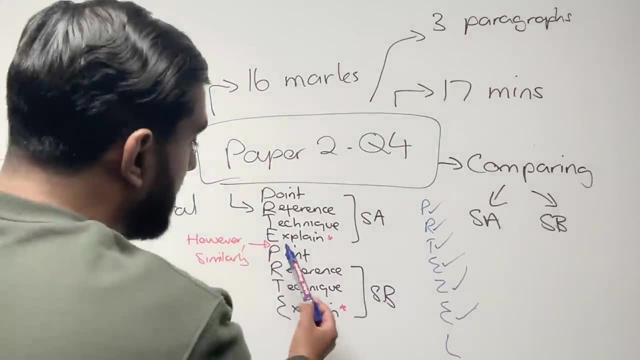 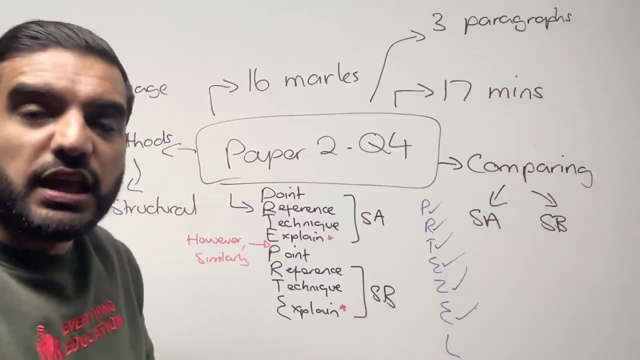 guys, the only thing that we're really adding is our point, because we're bouncing to the other source. Now, if your point is a similarity, have a very similar point. If your point is different, then of course, have a contrasting point. 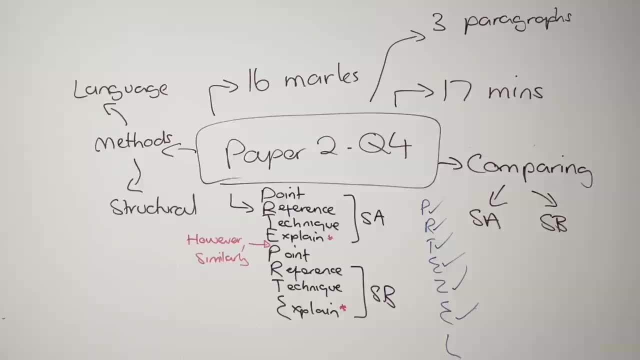 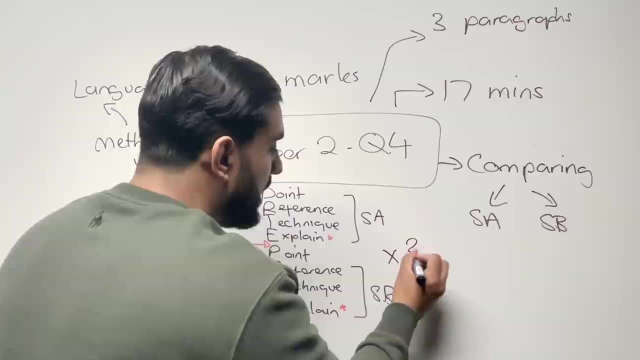 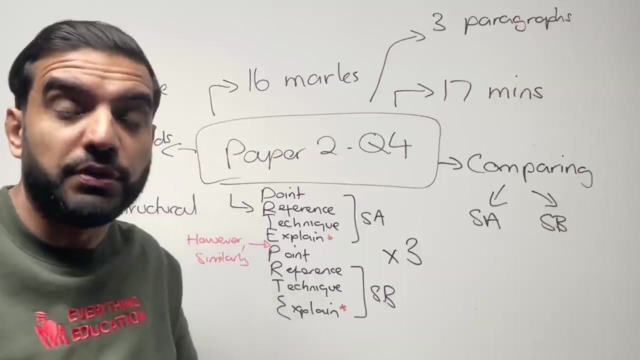 But, guys, the structure of the paragraph that we are aiming for is P-R-T-E, P-R-T-E, and this will be times three, because we are aiming for three paragraphs. Now I'm gonna prove to you, guys, where this structure was born from. 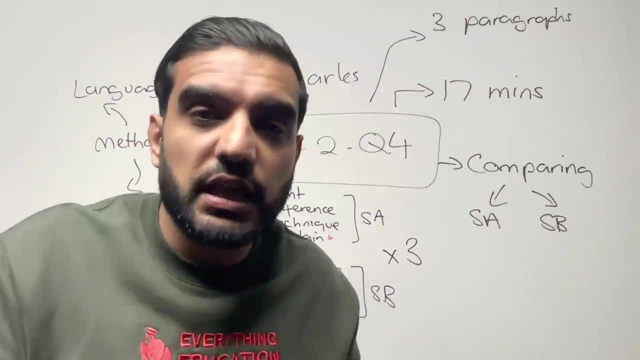 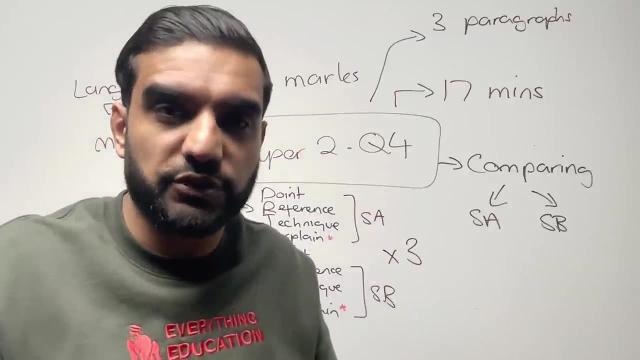 because this structure, guys, I didn't just one day pluck it out of the sky. It was born from the question, because, in the question, AQA tell us how to build the structure of this question. So, guys, now let's switch over to the question. 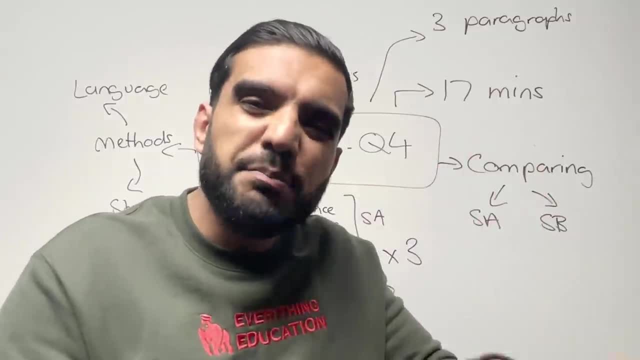 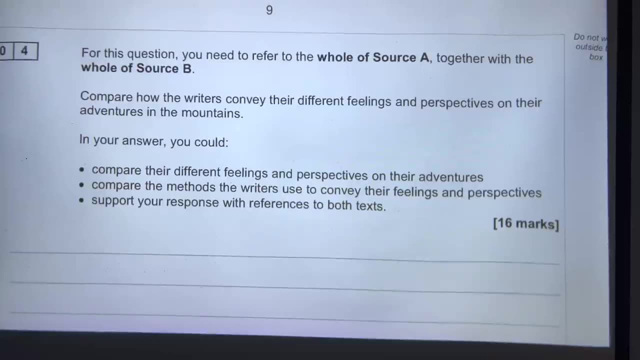 Let's go over the question, let's plan an answer and maybe we'll write one comparative paragraph. For this question, guys, we must refer to the whole of source A and the whole of source B. That is what we are looking at. 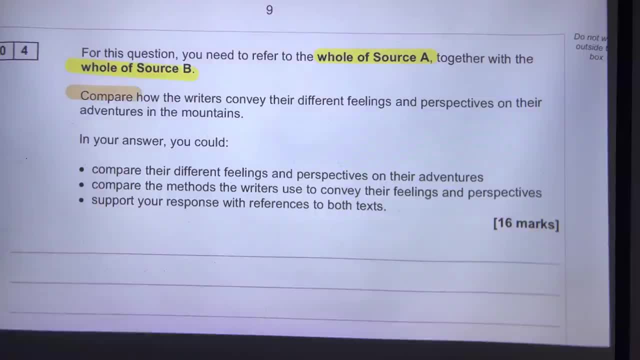 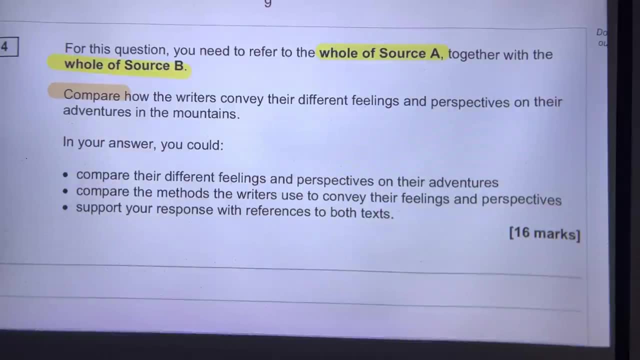 And instantly. guys, AQA is not shy, AQA does not hold back. They tell us from the very beginning: we want you to compare. Now, what are we comparing? We're comparing how the writers convey. convey is another word for show. 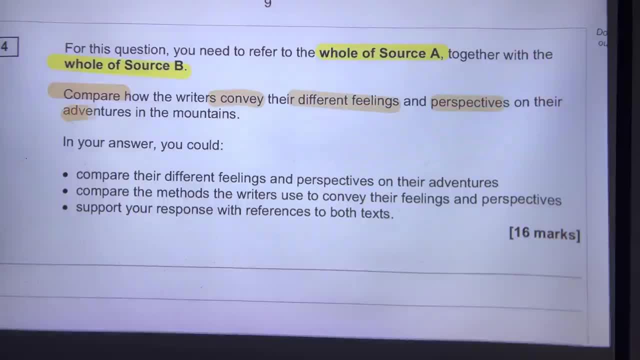 their different feelings and perspectives on their adventures in the mountains. Now, perspective, guys, it basically means their views. So how do the writers convey their feelings and their views about their adventures in the mountain? Now, this is where we know what paragraph structure to use. 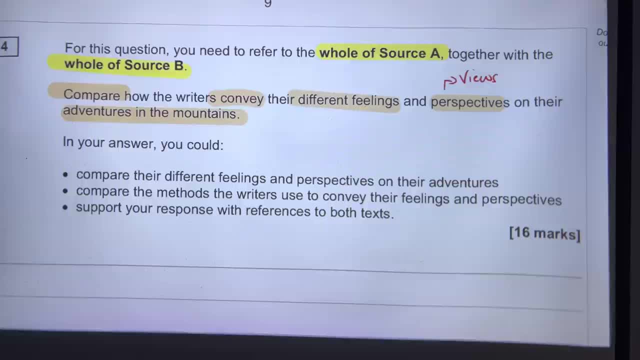 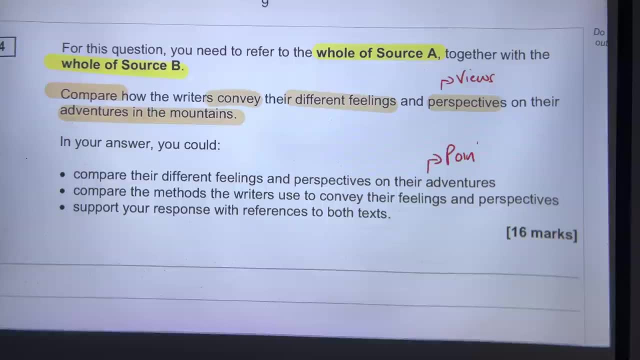 In your answer you could compare the feelings and perspectives of their adventures. Now, if I said that their adventures were terrifying in the paragraph, this would go down as my point. The third bullet point says: support this with reference to the text. 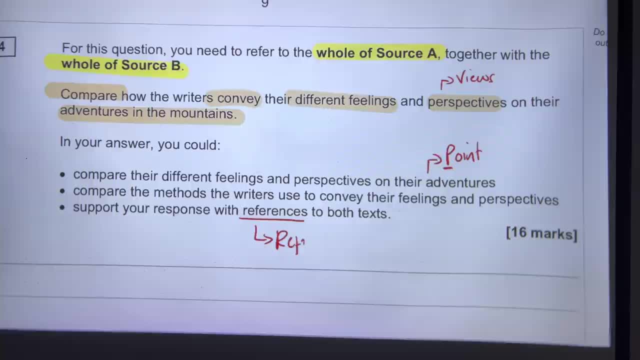 Now, when it says reference, we know it's talking about quotes. So this is the second part of the paragraph. So we have to have a point and we have to have a reference. Then it says: look at the methods, compare the methods. 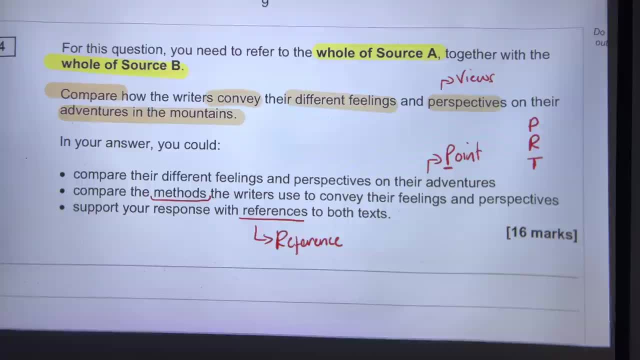 Now we call methods, or I call methods techniques. These techniques can be used to compare methods, methods, methods, methods, methods, methods, either language or structural techniques, and every time we talk about a technique we have to explain the effect. that is why, guys, i said to you guys earlier, we are doing point reference technique. 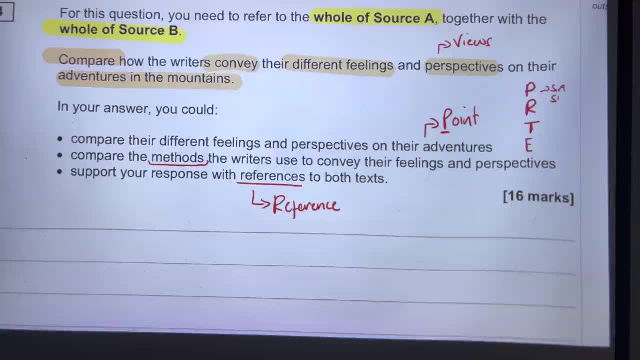 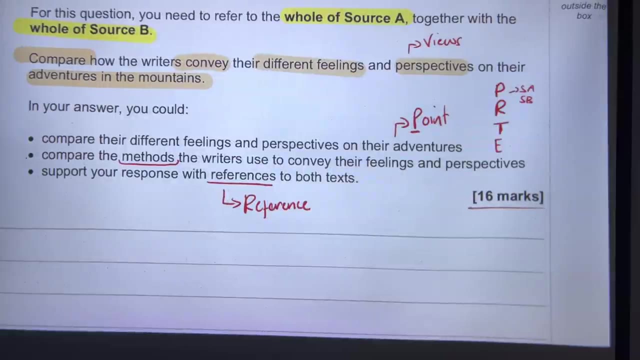 explain the effect for source a and source b, and that is where the paragraph structure comes from. and we know, guys, the 16 mark question. we are spending 17 minutes and we are looking to write three paragraphs. so what we're looking at, guys, we're looking at how they convey their different 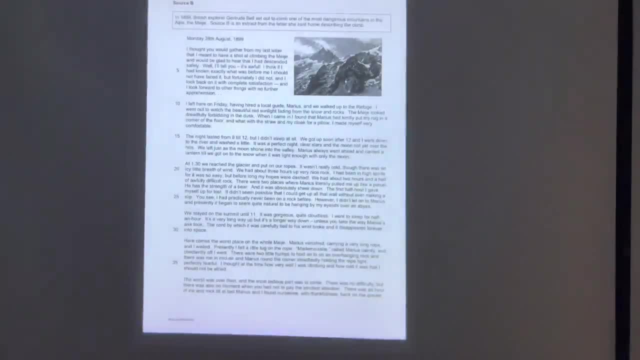 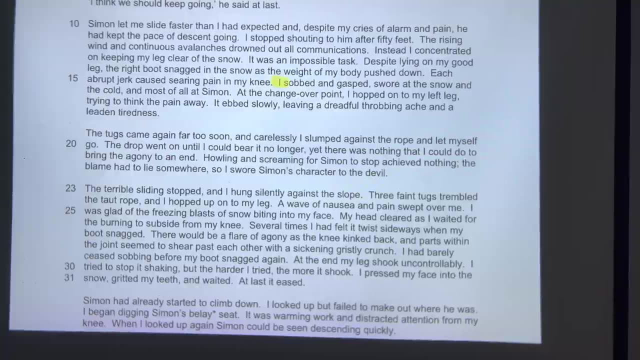 feelings and perspectives about their adventures in their mountain source. a. let's have a look at this part over here where it says: i sobbed and gasped, swore at the snow and the cold, and, most of all, simon. now this here guys, will be my reference, my technique that i will be talking. 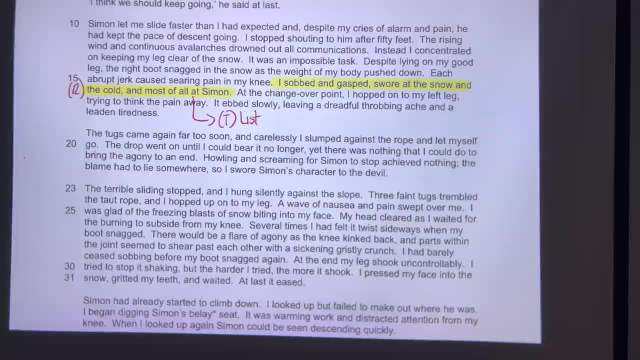 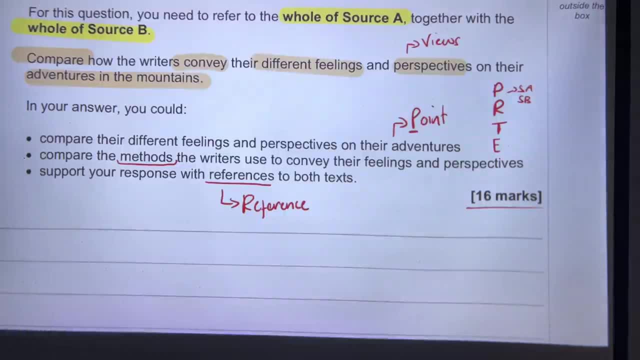 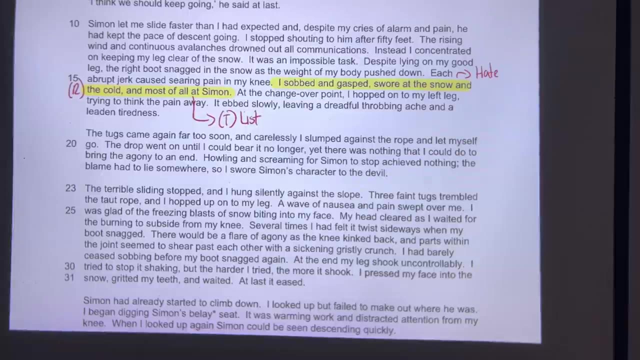 about here, guys, will be a structural technique of a list, and what will be my point, guys? my point will be: what was the question, guys? let's recap about the adventures in the mountain. this character i hated, absolutely hated the adventures in the mountain. i don't know why i shouted hated. but here we are, guys, so i've got my p. 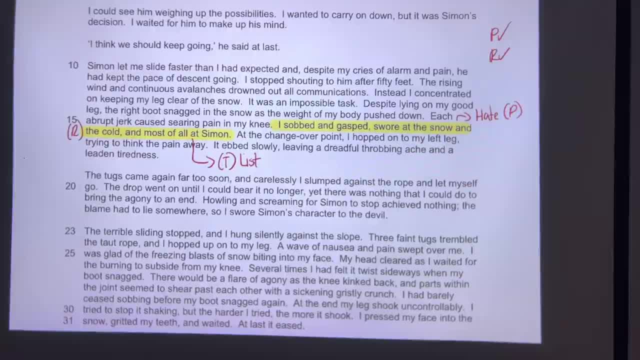 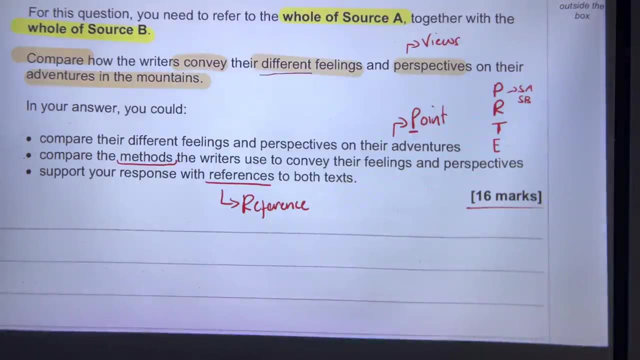 i've got my r, i've got my t and i will explain the effect when i begin writing my paragraph. so we are compared, we are comparing guys and we are making sure that we are looking at different feelings. so now, whereas in source a, i'm saying that this person absolutely hated it. 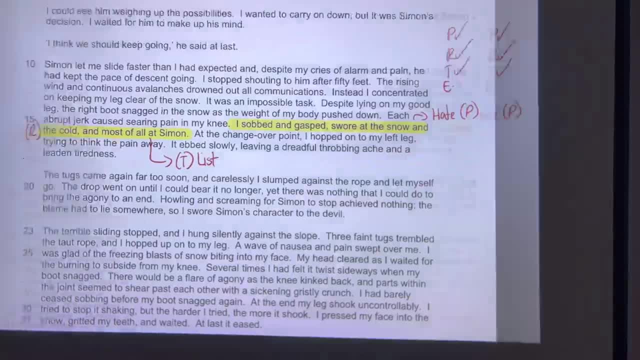 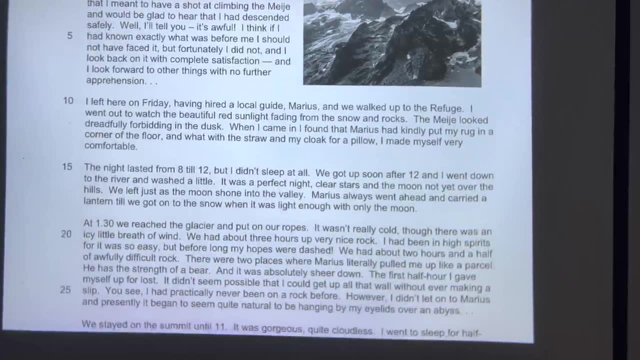 and i'm doing this via the structural device of a list. now i've got a look at source b and look at a method that the writer uses in this source to show us that this character um somewhat loved their experience, and i can see one staring right at me. guys. 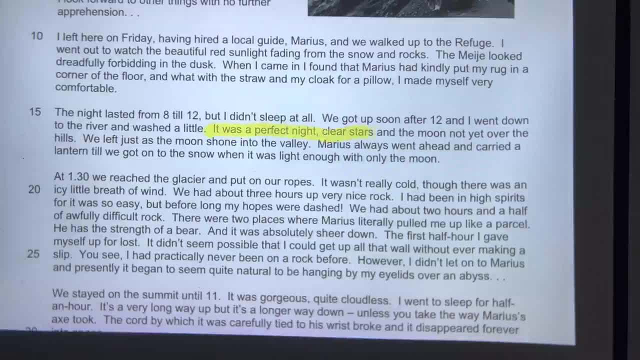 and i hope you can see it with me. it was a perfect night: clay stars and the moon- perfect, it was a perfect night: clay stars and the moon. now, this will be my reference. now, what technique has the writer used here? the writer here, guys, has used a rule of three, whereas in the first one there is: 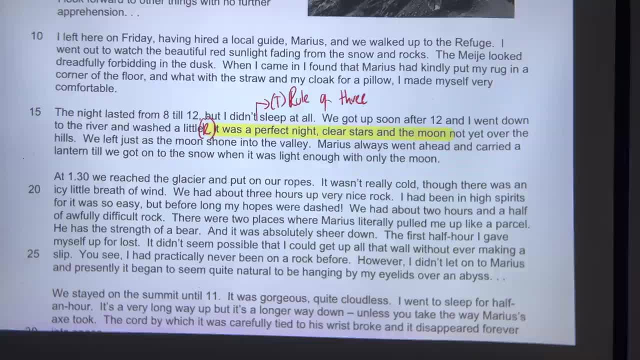 a list because it goes beyond three. here we get, we, we we stop at the third: perfect night, clear stars and the moon. rule of three guys, our reference, and how does this person view their experience? whereas in source a they hated it, this one loves it, absolutely loved it. um, that is the difference between the two. so that is my oops guys. 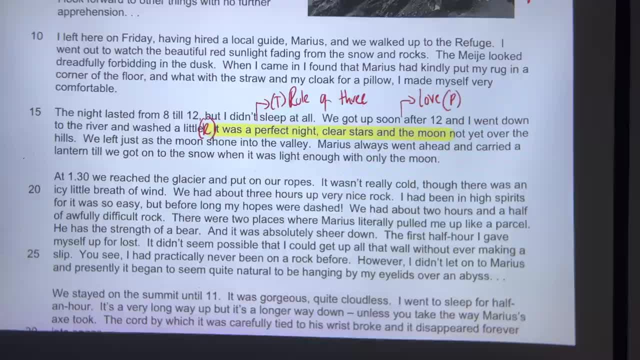 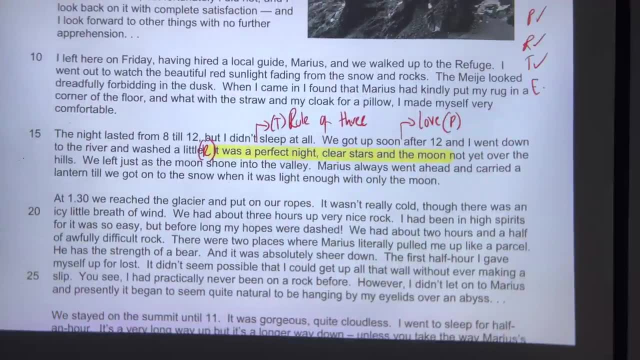 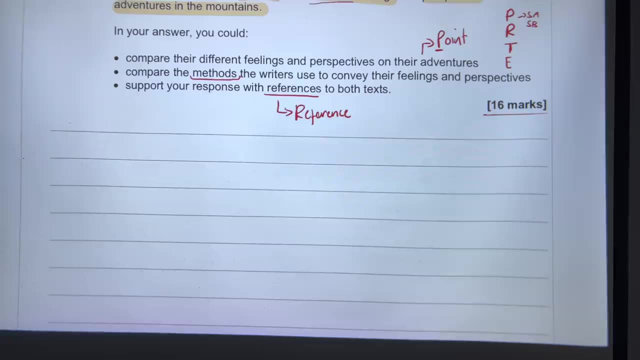 that is my point. so i've done my p, i've done my r, i've done my t, and i will do my effect later. now what i must do is turn these into one paragraph. the writer in source a absolutely hated the experience in the mountain, whereas 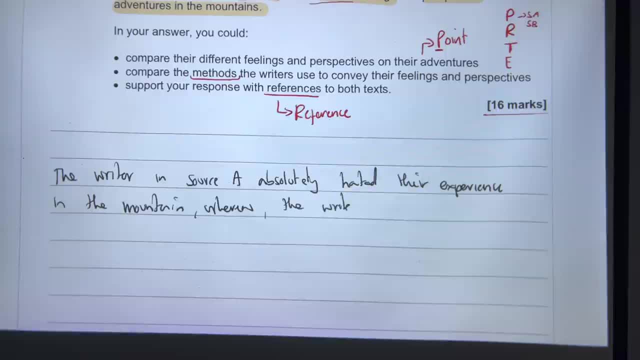 the writer in source b was the opposite. they loved it. and there is my quick point. and now let's move on to my reference. how much am i quoting? i won't quote the whole thing, i'm just going to quote the whole thing, things i'm going to refer to, the lines: 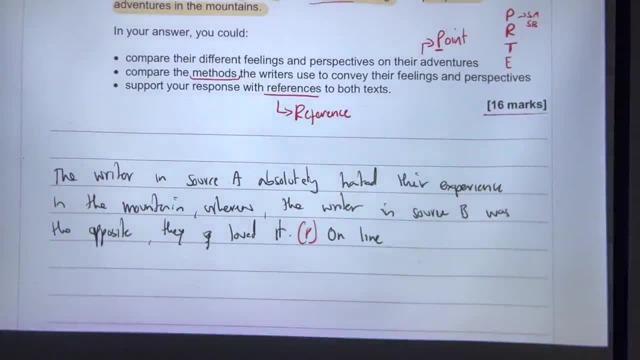 the whole thing, guys. i'm going to refer to the lines on lines 15 to 16 of source a. here, guys, we have a technique. sorry reference guys. here we have my reference. online's fitness is, you know, sauce a. the writer uses the writer 58 Запompka了. 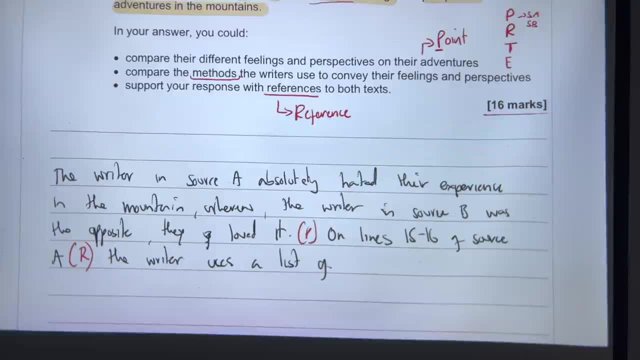 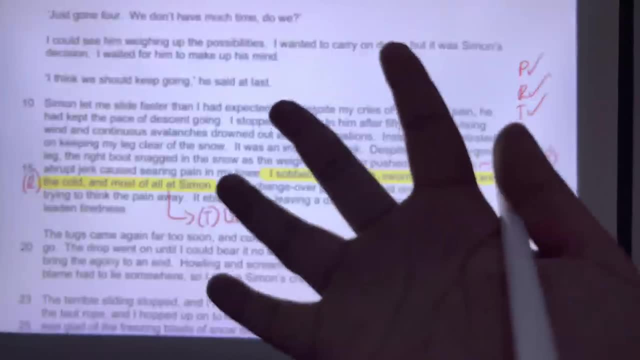 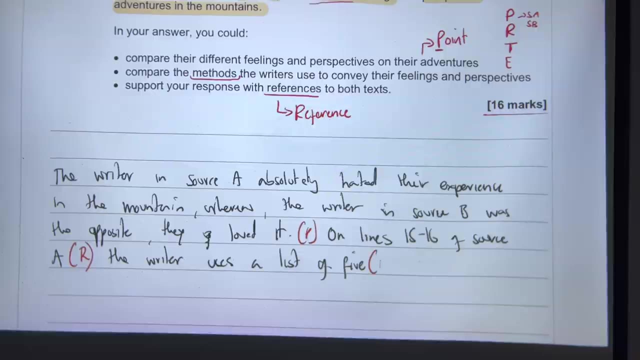 uses a list. the writer uses a list of. of how long is our list? I sobbed, I gasped, I swore at the snow, at the cold and, most of all, Simon 5.. We have a list of 5.. The writer used a list of 5.. That is my technique. Now, guys, if you 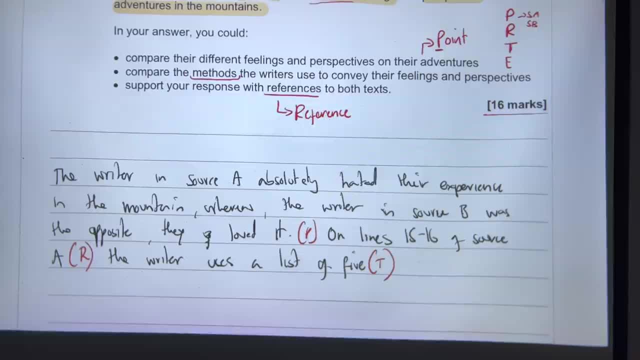 ever. guys, if you ever use a list in your exam, try to be specific, the way I am, Try to tell the examiner how long your list is. So I've done my P, I've done my R and I've done my T. Now let's. 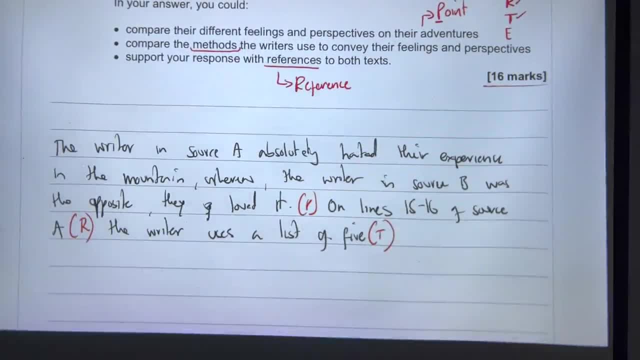 have a read, guys. The writer in source A absolutely hated the experience in the mountain, whereas the writer in source B was the opposite: They loved it. On lines 15 to 16 of source A, the writer uses a list of 5.. Oops, Now what is important about the list of 5?? 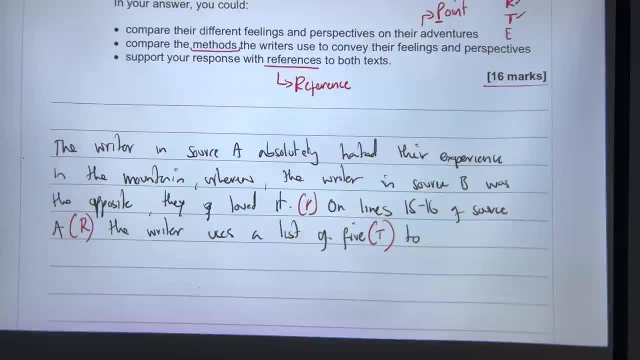 It could have been. the writer could have said: I sobbed full stop or I gasped full stopped. but because the writer says I sobbed and I gasped, and this and this and this, it makes it clear that this is a never-ending experience. This is a never-ending ordeal. It goes on and on and on. I was about to. 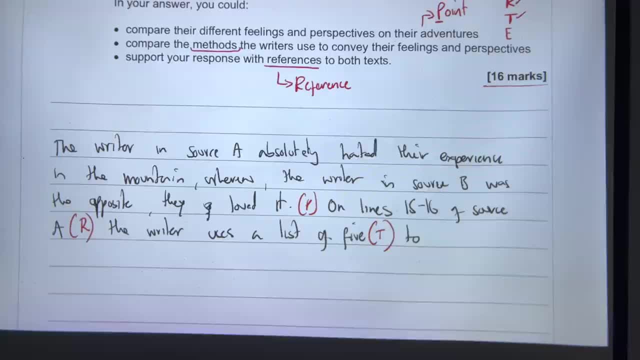 burst into a song there. but let's not do that, and that is what I want to make clear here, guys. The writer uses a list of 5. To emphasize how the torture they suffered on the mountain was never ending. It was one ordeal followed. 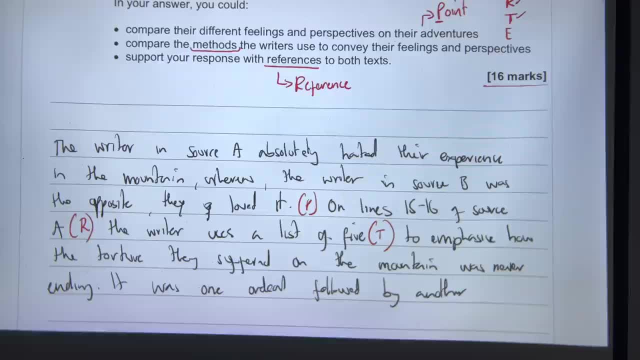 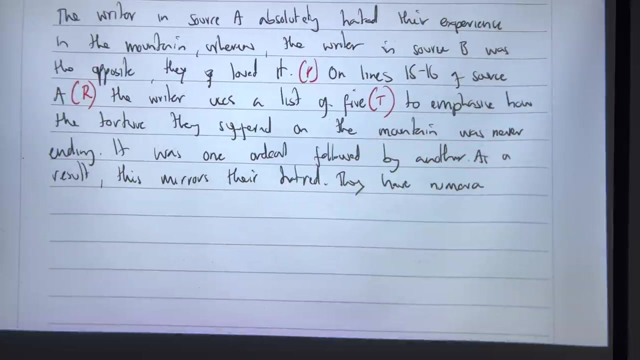 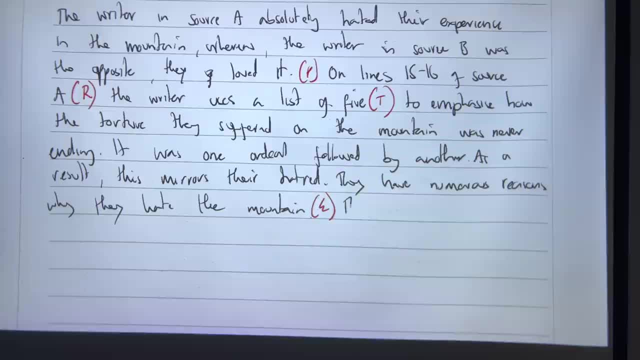 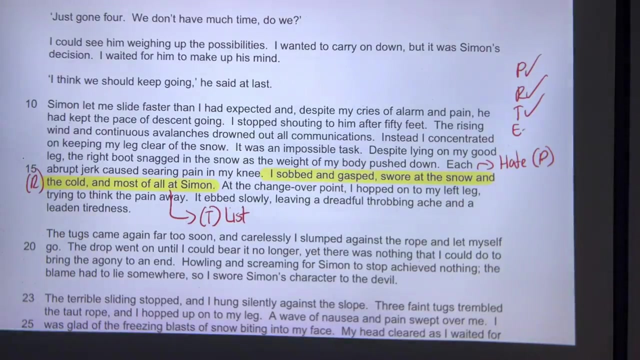 back later. I'm going to bounce back. This feeling of hatred contrasts the love displayed in the. This feeling of hatred contrasts the love displayed in the. This feeling of hatred contrasts the love displayed in the source B, In Source B, In Source B. 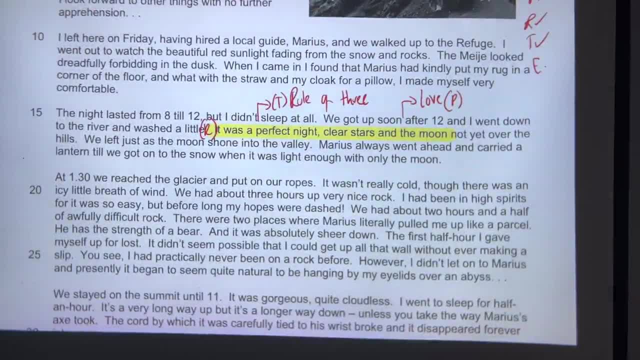 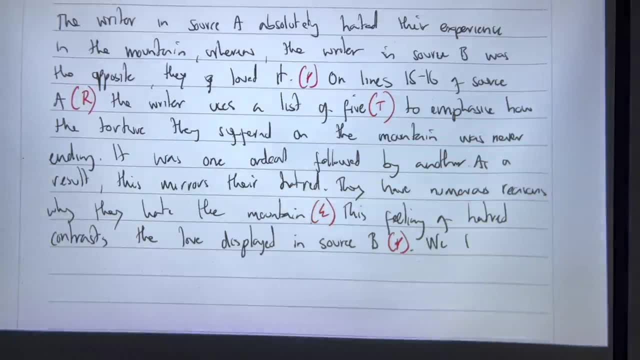 That's my point. That's my point. That's my point, What's my take, What's my reference. We learn how, know how to. it was a perfect night, clear stars and the moon. that's my reference, guys, that's my reference. now i give my technique. 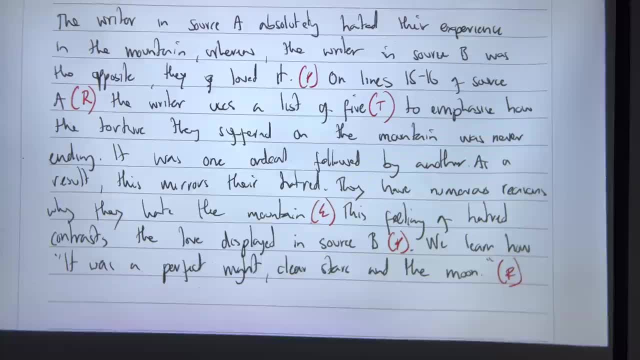 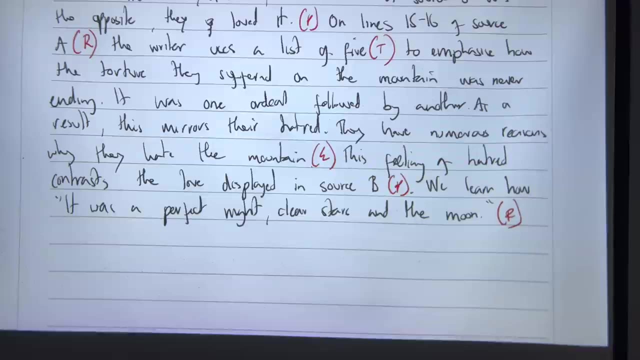 this feeling of hatred contrasts a love display. in so speed we learn how it was: a perfect night, clear stars and the moon. and now i begin, the subtle references back and forth. just subtle references, guys. why a list is used in source? a a rule of three is used in source. be to have the. 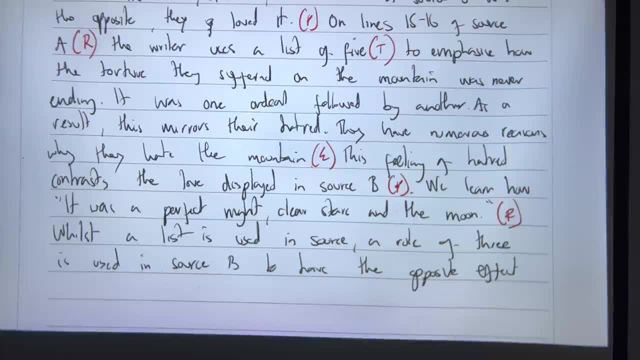 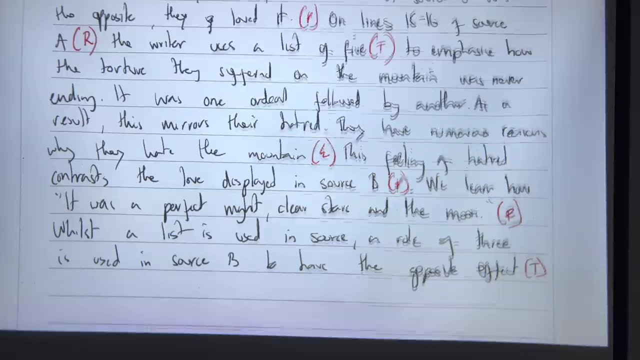 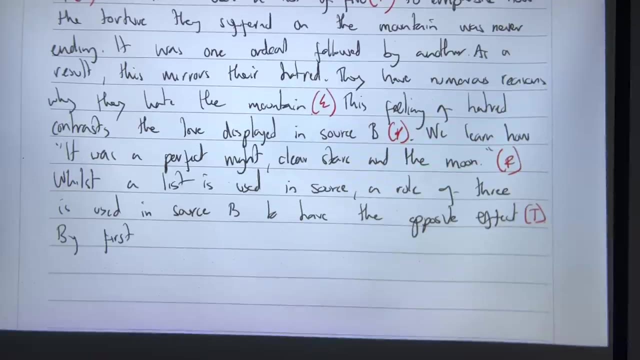 opposite effect. and that's me just mentioning my technique, guys. and now let's explain what this tech, what this effect is by first, where's the call, guys, where's the call? by first mentioning the night and then using the rule of three to zoom in to the beautiful. 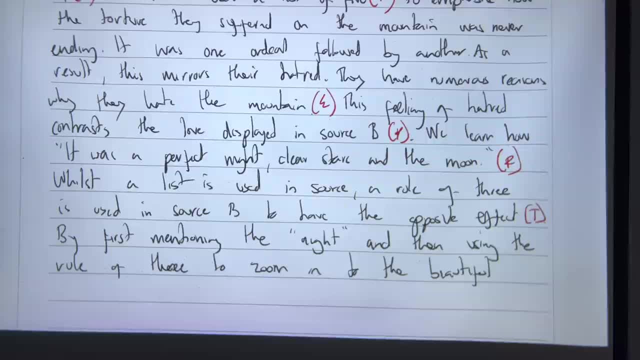 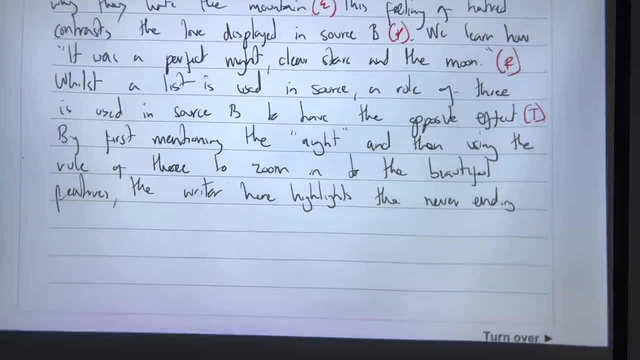 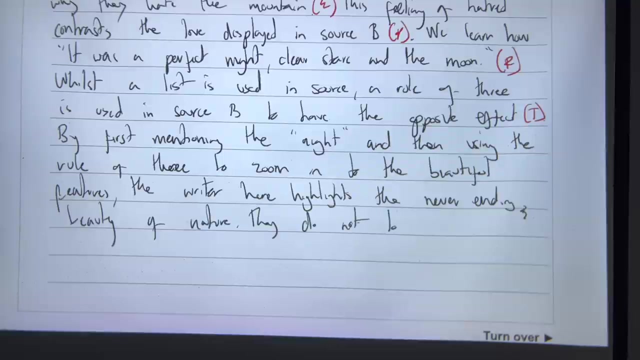 features the writer here highlights and the never ending beauty of nature. they do not love it for one reason. let me change nature to mountain. let me change nature to mountain of the mountain. they don't love it for one reason: they love it for multiple. all right, guys, then i insert my summative comment. as a result, both writers use similar techniques. 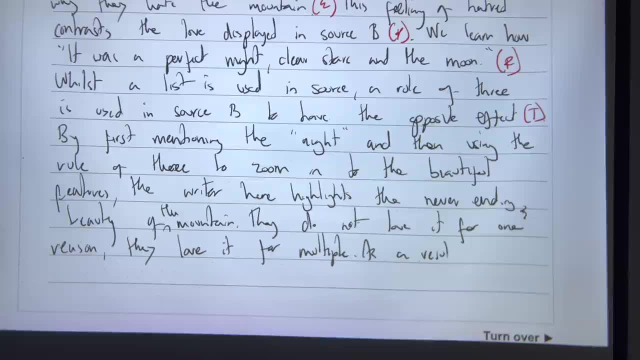 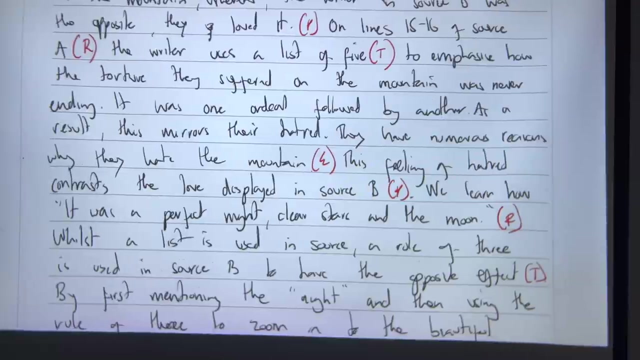 as a result, both writers use similar techniques, techniques. both writers use similar techniques, techniques to display the contrasting views of the mountain. all right, guys. that is an example of a pre paragraph. i begin here, guys, with my p, then my r, then my t and my e, then i bounce across p, then i bounce around here. 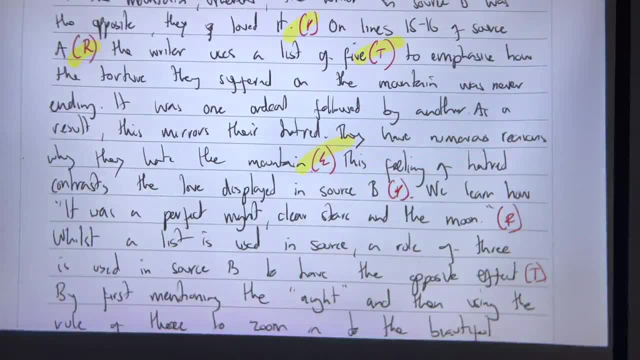 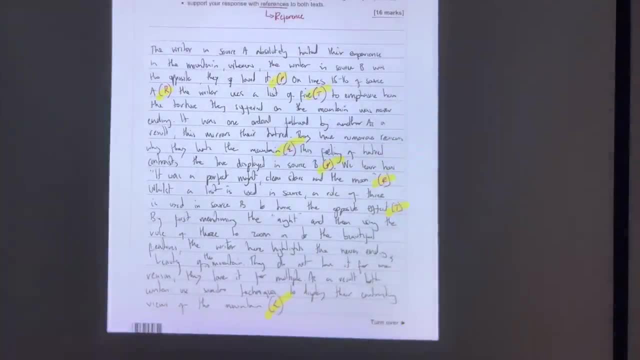 once again. let's go to this book. let's jump in here and look at this paragraph, a paragraph in a paragraph. here, guys, this is an singers book- r, t and e- and that is an exemplar paragraph that i've written myself. the writer in source a. 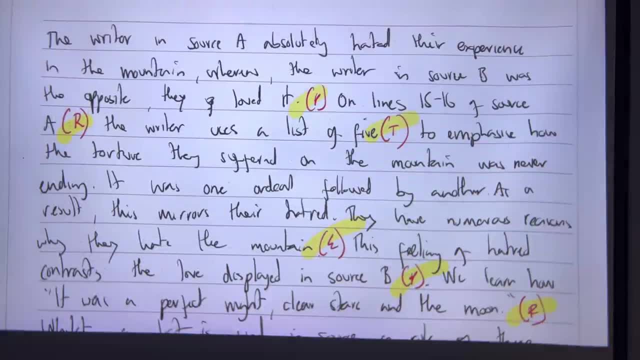 absolutely hated the experience in the mountain, whereas the writer in source b was the opposite: they loved it. on lines 15 to 16 of source a, the writer uses a list of five to emphasize how the torture they suffered on the mountain was never ending. it was one ordeal followed by another. 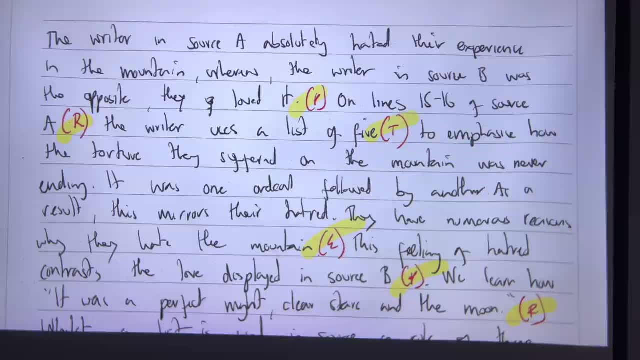 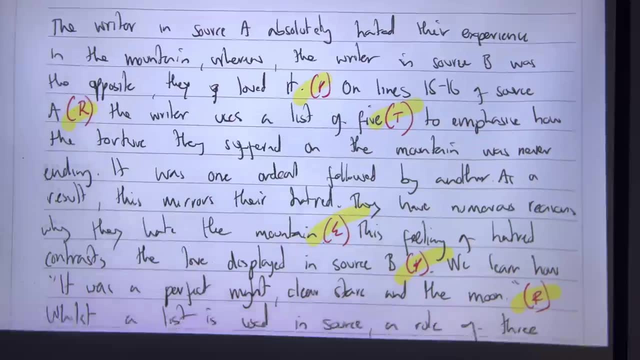 as a result, this mirrors their hatred. they have numerous reasons why they hated or why they hate the mountain. this feeling of hatred contrasted love, displayed in source b. we learn how it was: the perfect night, clear stars and the moon, with a list or with a lip, whilst the list is used in 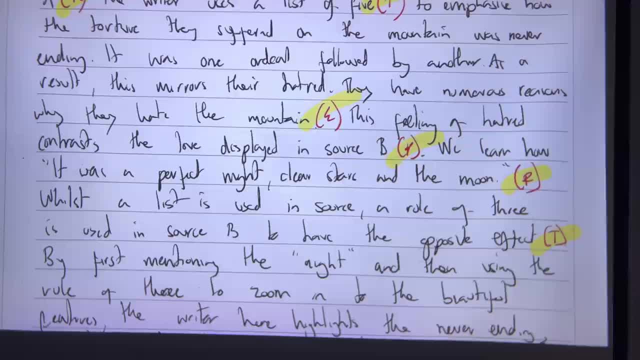 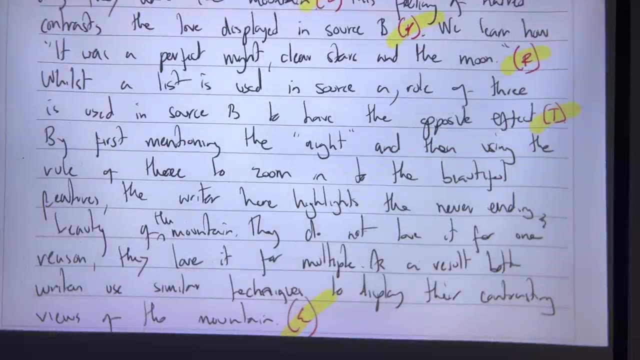 source a. i don't know why there's a comma here. while the list is used in source a, rule of three is used in source b to have the opposite effect, by first mentioning the night and then using the rule of three to zoom in to the beautiful features. the writer here. 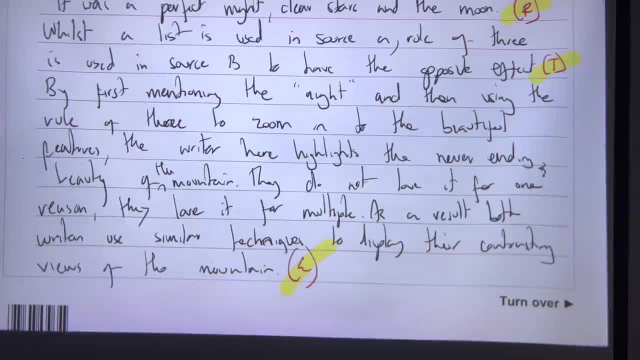 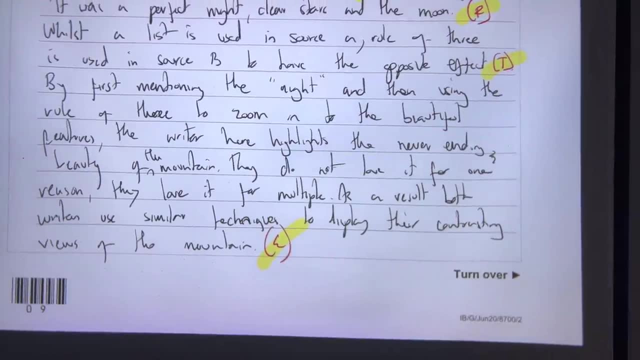 highlights the never-ending beauty of the mountain. they do not love it for one reason: they love it for multiple. as a result, both- both- both writers- use similar techniques because a list and a rule of three guys, they're very similar. rule of three is three, list is anything more, and in this case we